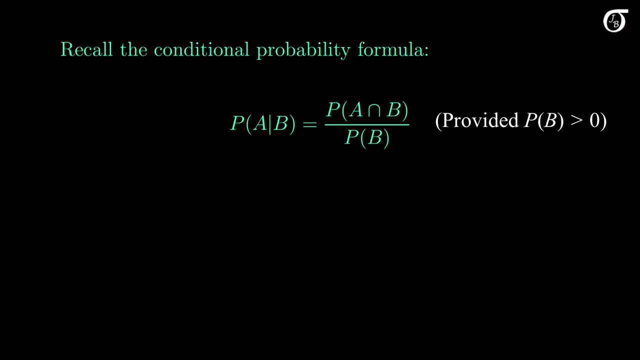 if the probability of the event we are conditioning on is greater than zero. This isn't a problem in practice, as we don't typically have an interest in conditioning on events with zero probability. I'm not going to discuss that restriction in the formulas that follow. 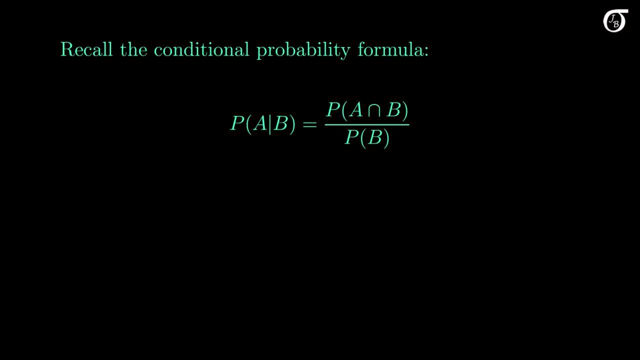 but that is always an underlying mathematical restriction in conditional probability. Also, recall that if A and B are independent, then the probability of A given B is equal to the probability of A. In other words, the knowledge that B occurs does not change the probability of A. 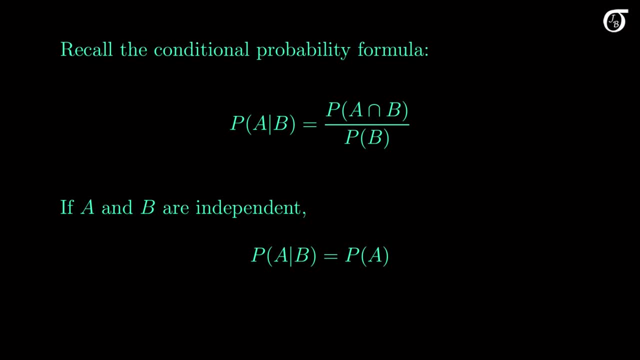 Which event we call A and which we call B is arbitrary, so we could switch the roles of A and B in these formulas. I go into much more detail about conditional probability and independence in my videos on those topics. In the two-event case like this: 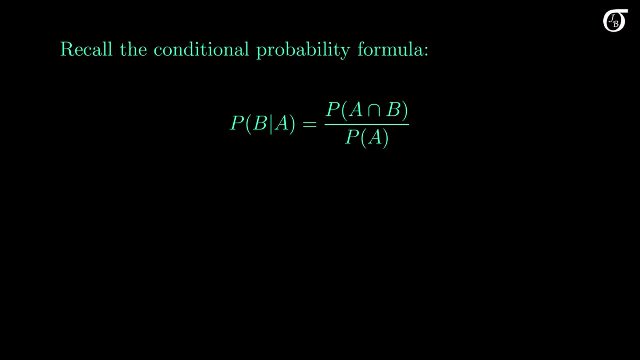 the multiplication rule simply reworks this conditional probability formula, isolating the probability of the intersection by bringing the denominator to the other side. Let's see what that looks like. Here's the multiplication rule for two events. We'll generalize this to more events later. 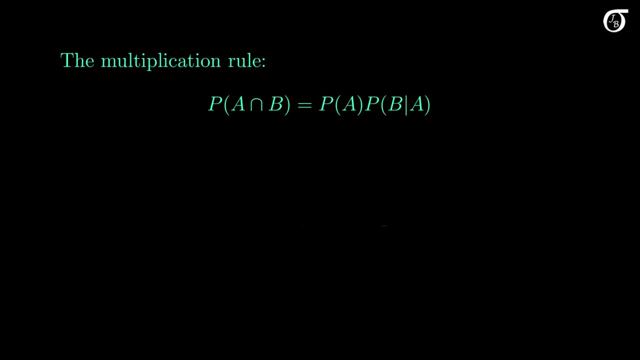 The probability of the intersection of A and B is equal to the probability of A times the probability of B given A, And we can, of course, switch the roles of A and B. The probability of the intersection is also equal to the probability of B times the probability of A given B. 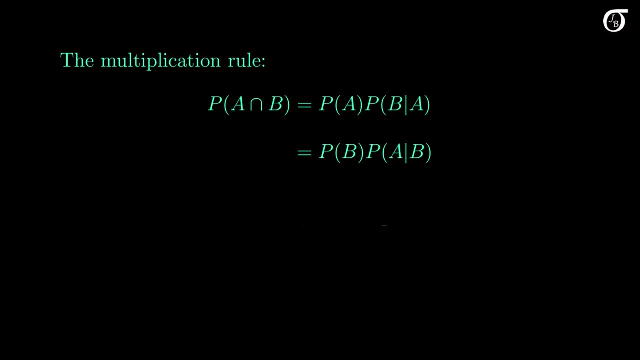 I think this makes intuitive sense. If we want the probability of A and B, we take the probability of one event and multiply it by the conditional probability of the other, given the first occurs. And if A and B are independent, then the probability of A given B equals the probability of A. 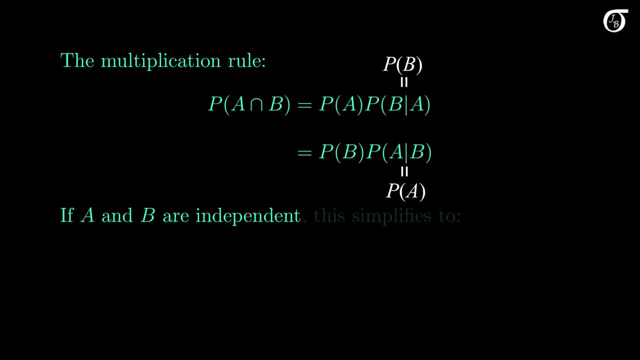 the probability of B given A equals the probability of B, and the multiplication rule simplifies to this. The probability of the intersection of A and B equals the product of the individual probabilities. Remember again, this last statement is true if, and only if, A and B are independent. 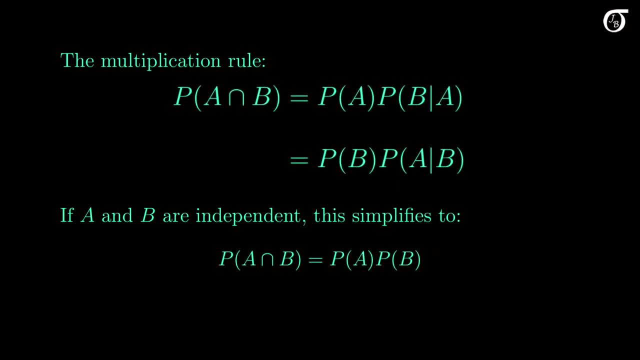 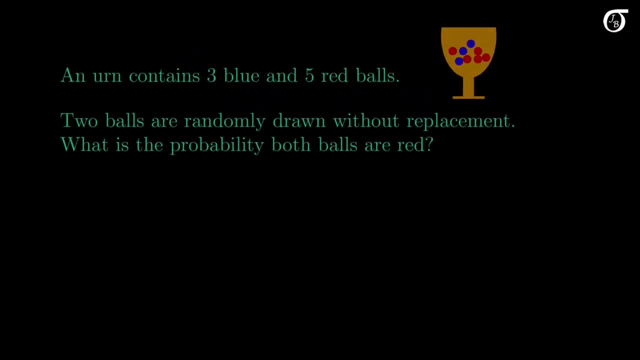 whereas the multiplication rule up here holds in general. Let's work through a simple example. An urn contains three blue and five red balls. You might think that looks a little more like a goblet, but I'm calling it an urn and sticking to it. 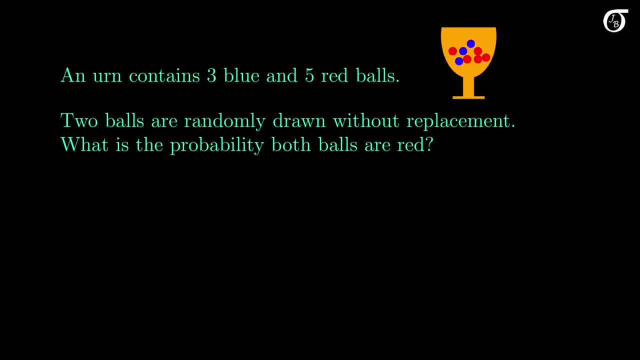 Two balls are randomly drawn without replacement. What is the probability that both balls are red? Let's call event A, the event the first ball is red, and event B, the event the second ball is red. We want to find the probability both balls are red. 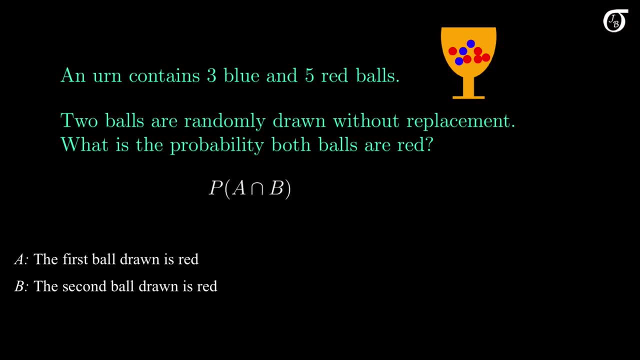 or in other words the probability of the intersection of A and B. We'll find that with the multiplication rule, multiplying the probability, the first ball is red. by the conditional probability, the second is red. given the first is red, We could try to do this the other way around. 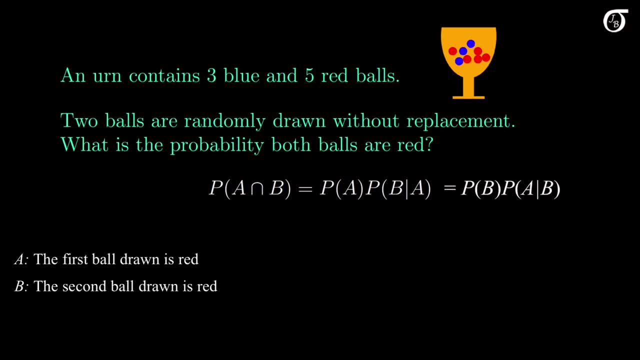 multiplying the probability, the second ball is red times the probability, the first is red, given the second is red, And while that works out to the same thing, it's trickier to think about, And here it's much more natural to go in order. 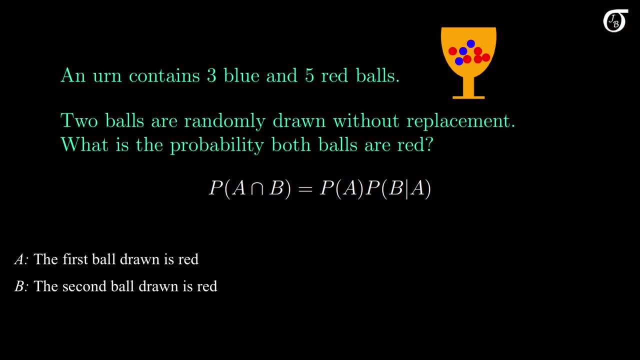 putting the first ball drawn first, then, conditioning on that outcome On the first ball, we're randomly picking one ball from eight, where each ball is equally likely to be picked. There are five red balls, so the probability of getting a red ball in the first draw is 5 out of 8.. 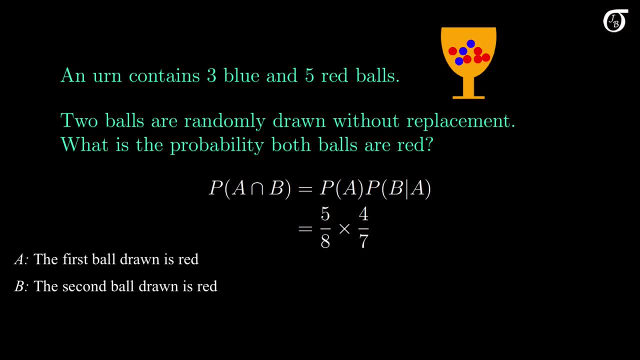 If the first ball is red, then there are only four red balls in the seven remaining balls, since we're drawing without replacement. So the probability of getting a red ball on the second draw, given the first ball was red, is 4 out of 7.. 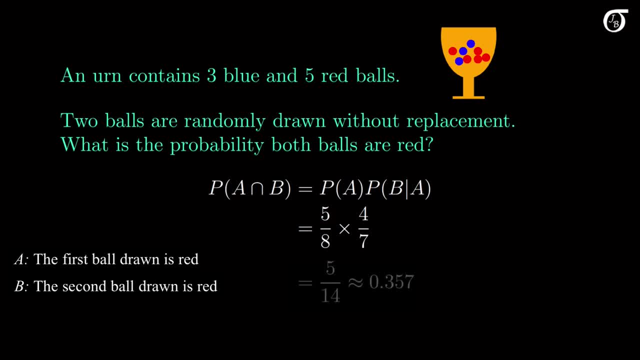 If we multiply that out, we get 20 out of 56, which reduces to 5 out of 14, or to three decimal places: 0.357.. Here's another example. Suppose the probability of A is 0.4,. 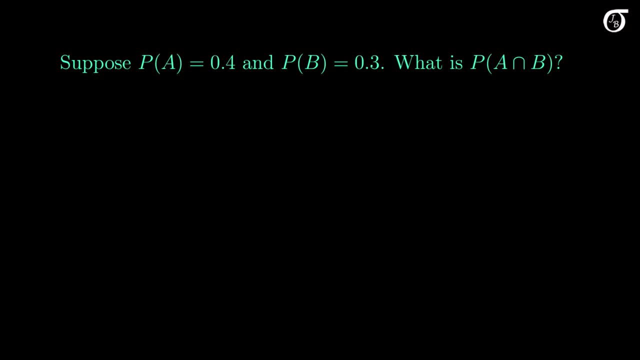 the probability of B is 0.3, and we want to know the probability of their intersection. This one is quick to answer, because it cannot be answered. We can't find the probability of the intersection from only the individual probabilities. Now it might be tempting to say 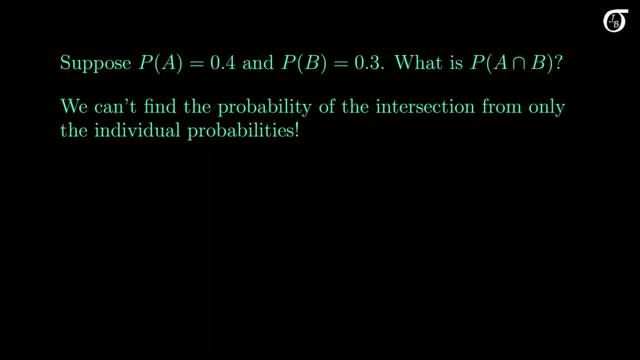 hey, we just learned the multiplication rule. let's just use that. It's not going to work, but let's try it. Here's the multiplication rule. First, recognize that we don't have the probability of B given A, and there's no way to get it here. 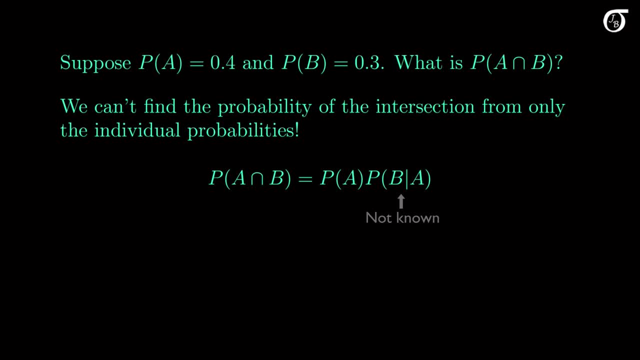 We can't get the probability of A given B either, so we're stuck. But we might try to get clever and recognize that the probability of B given A is the probability of the intersection of A and B over the probability of A. Then the probability of A cancels. 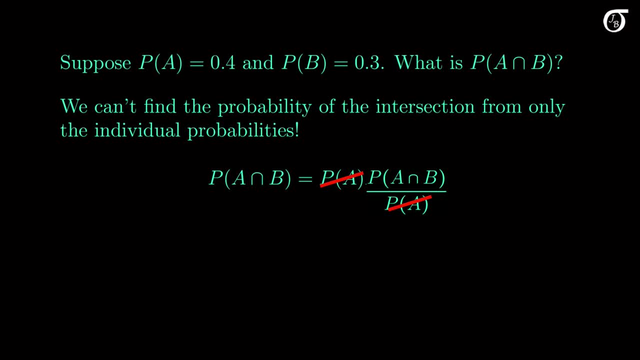 and we're left with the notion that the probability of the intersection of A and B is equal to the probability of the intersection of A and B. While true, that's not an especially useful notion, We're just spinning our wheels here, going around in circles. 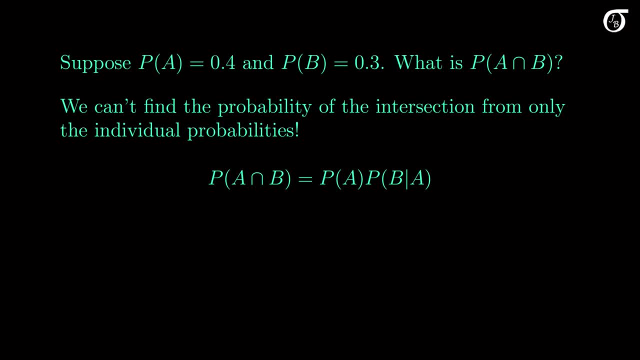 What I'm getting at is that the multiplication rule is true in general, but that doesn't mean it's always helpful to find the probability of the intersection. We can't find that probability here. There simply isn't enough information. We would need another piece of information. 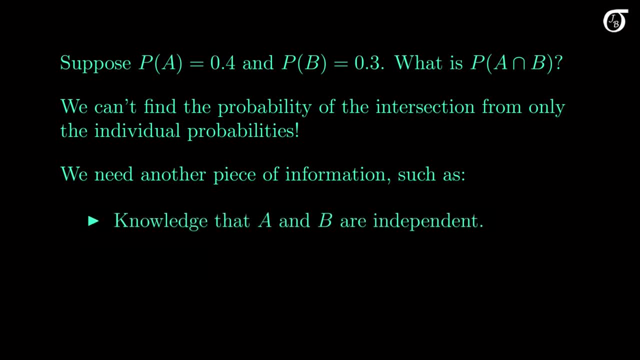 For example, the knowledge that A and B are independent, then the probability of the intersection is just the product of the individual probabilities, or perhaps the probability of the union of A and B. If we had that, then we could use the addition rule. 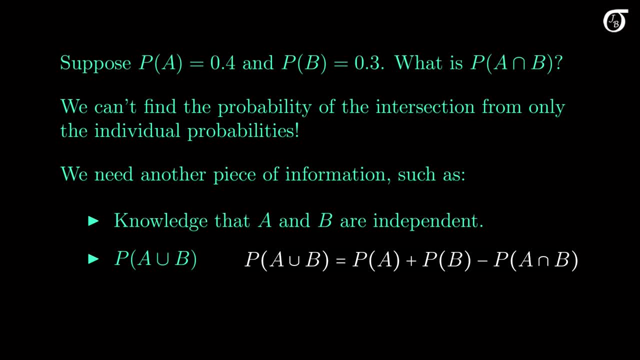 and isolate the probability of the intersection, as we would have the other three probabilities And there are other possibilities as well. But in any event we would need more information to find the probability of the intersection. So I'll warn you once again to not simply jam things into the nearest formula. 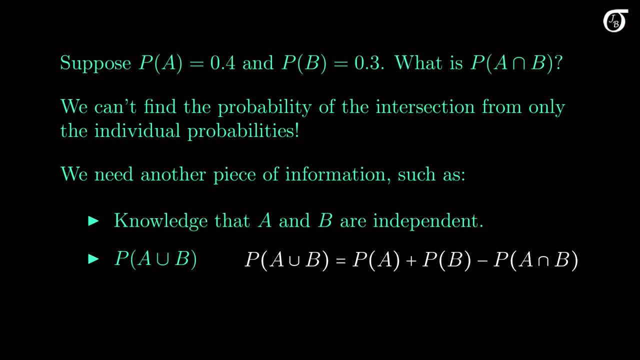 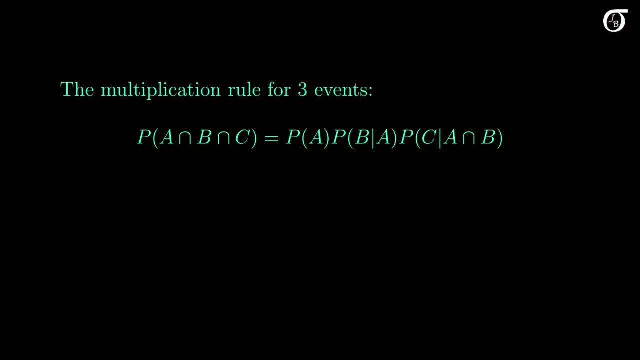 The formulas hold in general, but that doesn't mean they're always useful to answer a question. We've now looked at the multiplication rule for two events, but it also extends to three or more events. Let's have a look at that. Here's the multiplication rule for three events. 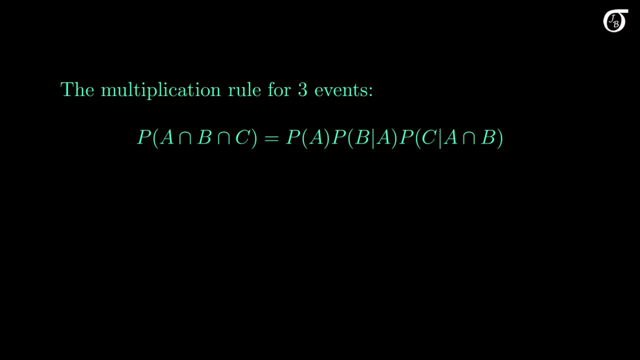 The probability of the intersection of A and B and C is equal to the probability of A times the probability of C. The probability of B given A times the probability of C given A and B. We could switch the ordering of A, B and C, of course. 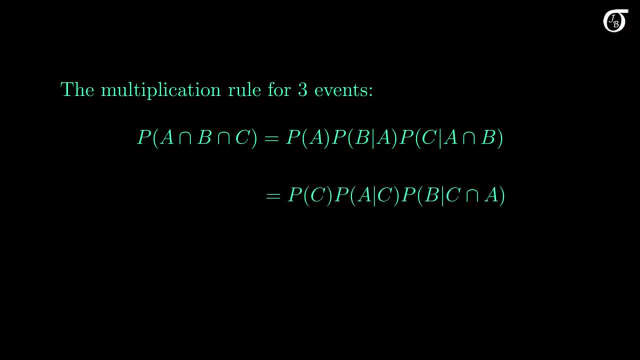 The probability of the three-way intersection is also equal to this, And there are four other orderings of A, B and C that we could write down if we really felt like it. In any event, we always start out with the unconditional probability of one of the events. 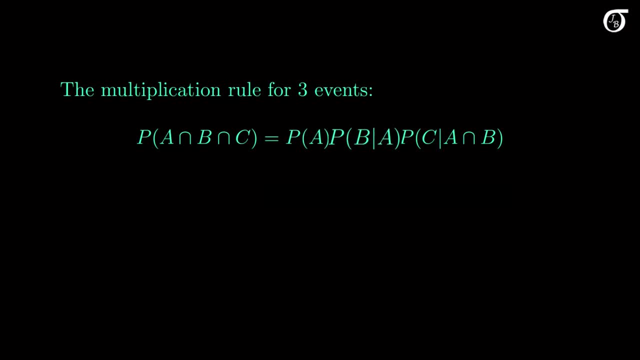 then multiply that by the conditional probability of another, given the first, then by the conditional probability of the third, given the first two, And this generalizes in a very natural way to any number of events. Let's work through an example. A Canadian is randomly selected. 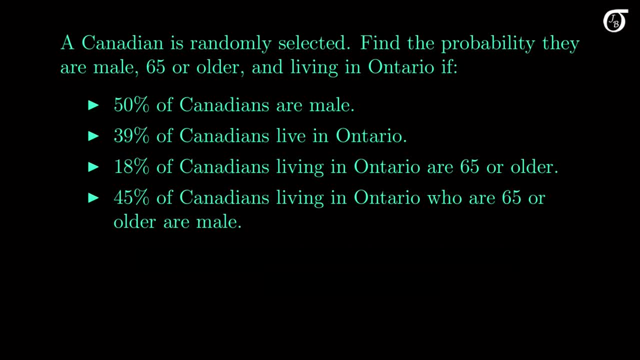 Find the probability they are male, 65 or older and living in Ontario. if we have the following information- All percentages are from Statistics Canada. using their definitions, The information we are given is that 50% of Canadians are male. It's actually a touch lower, at 49.7%. 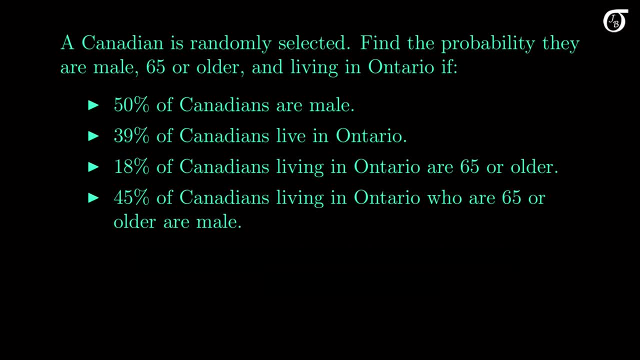 but I'm rounding everything to whole numbers here. I'll let M represent the event that the randomly selected person is male. so the probability of event M is 0.5.. 39% of Canadians live in Ontario. I'll let O represent the event that the randomly selected person lives in Ontario. 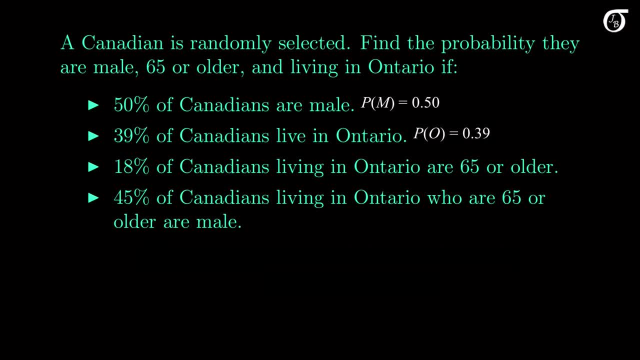 so the probability of event O is 0.3.. 39%- 18% of Canadians who are living in Ontario are 65 or older. I'll let E represent the event that the randomly selected person is 65 or older, that they are elderly. 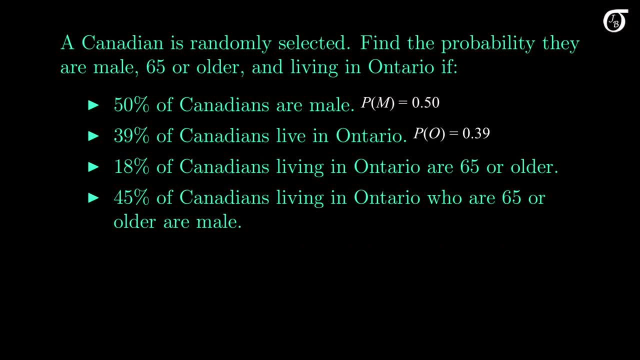 Here. we're told that 18% of Canadians living in Ontario are 65 or older. So the probability of E given O is 0.18.. Given they live in Ontario, the probability the randomly selected person is 65 or older is 0.18. 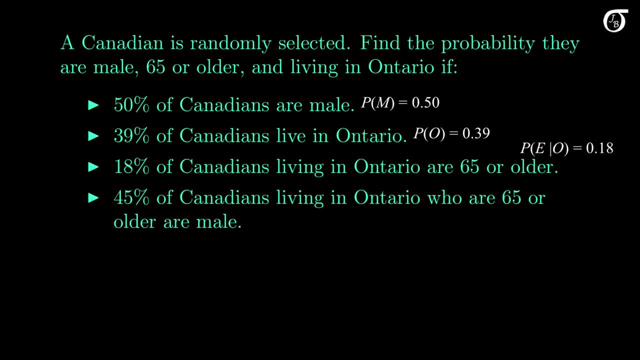 45% of Canadians living in Ontario who are 65 or older are male, And that means the probability a randomly selected person is male, given they live in Ontario and are 65 or older, is 0.45.. At older and older ages, the proportion of males tends to decrease. 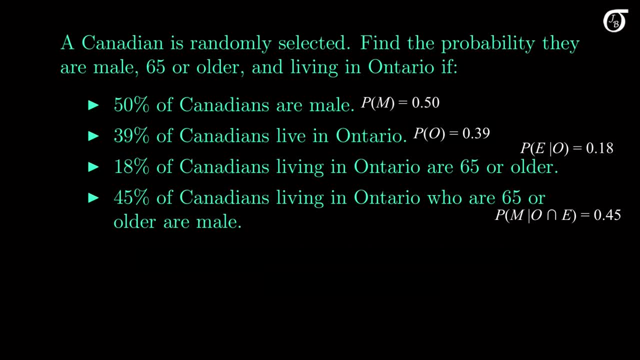 as males don't tend to live as long, We are asked to find the probability. the randomly selected person is male, lives in Ontario and is 65 or older. In symbols, that's the probability of the intersection of M, E and O.